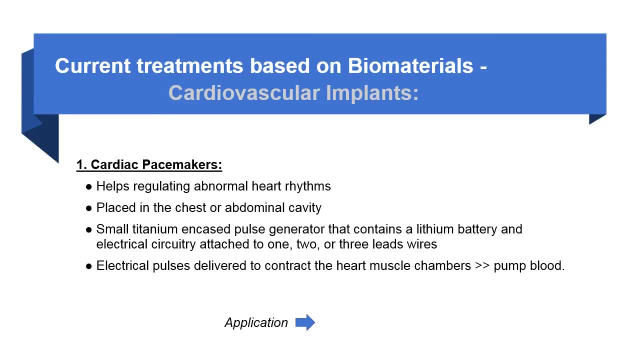 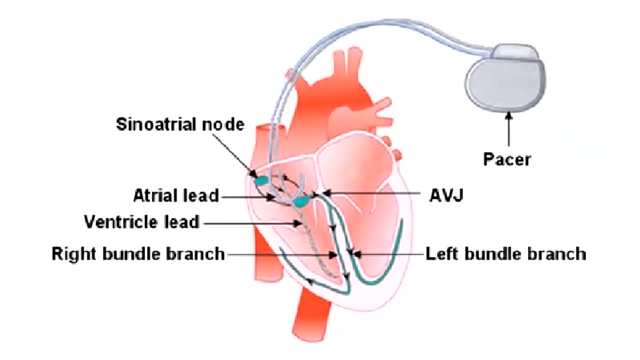 Cardiac pacemaker. Cardiac pacemakers are small. Cardiac pacemakers are small medical devices primarily designed for regulating abnormal heartbeats or to treat arrhythmia, and are placed inside the chest or abdominal cavity by surgical procedures. These devices consist of a lithium battery that is enclosed by a titanium case and has 1 to 3 electrodes. 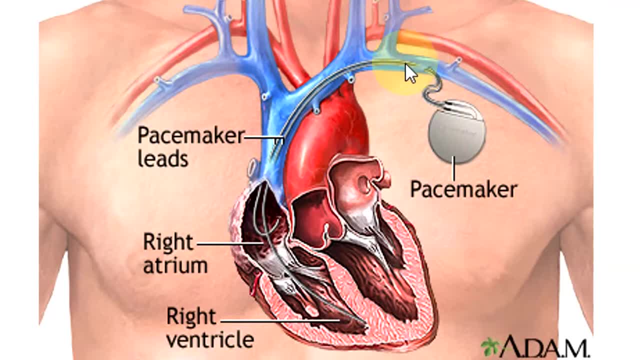 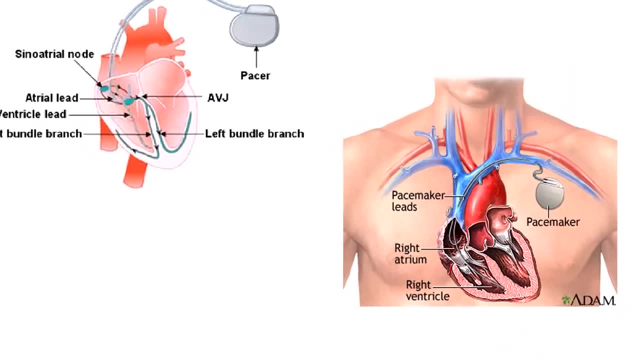 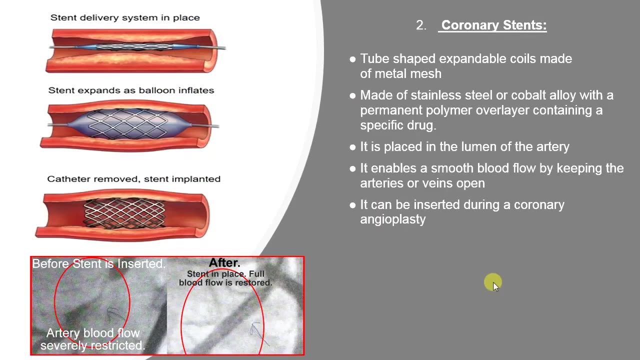 While operating, electrical impulses are being generated and sent through the leads to the heart chamber to stimulate the corresponding cardiac muscles for contraction and therefore pump blood. heart electrical conduction system Stents. Stents are tube-shaped metal mesh made of stainless steel or a cobalt alloy with a permanent polymer overlay containing a specific drug. 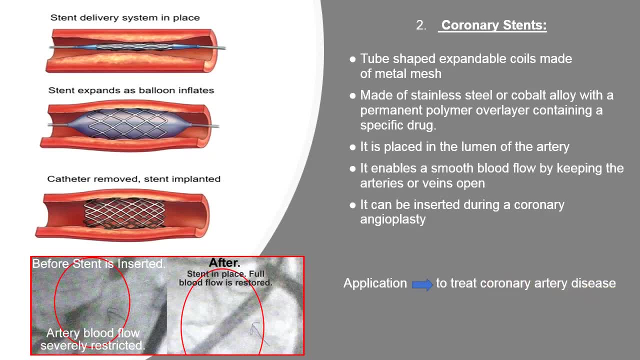 They are specifically designed for preventing coronary artery disease by being inserted into arteries via coronary angioplasty, as to enable a smooth blood flow by keeping the narrowed lumen open. The procedure is done by first threading a catheter, a thin tube, through a small puncture in a leg or an arm artery. 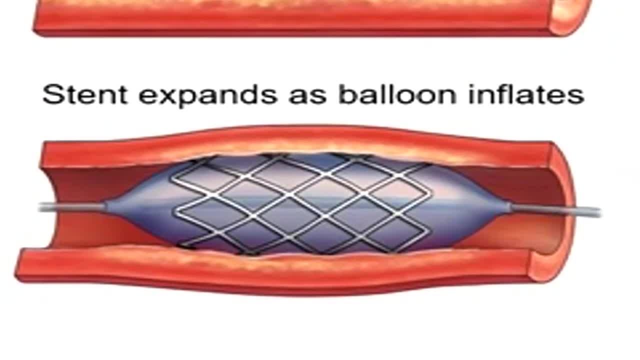 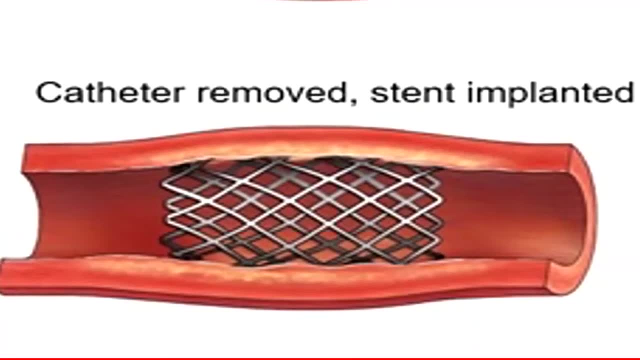 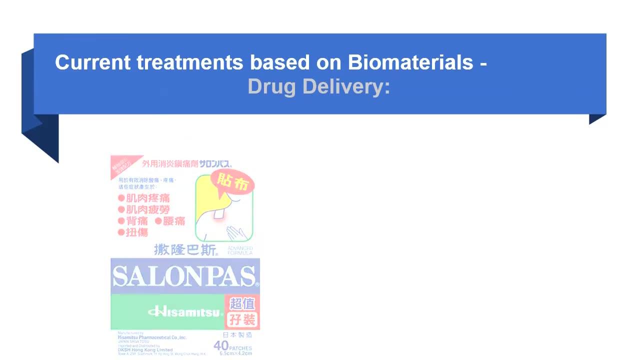 To the heart And secondly, inflating a tiny balloon region to open the narrowed artery. The insertion will finally be completed by placing the stents permanently within the inflated region. Drug delivery is another common biomaterial based treatment. The first application I will be talking about is the eye drops. 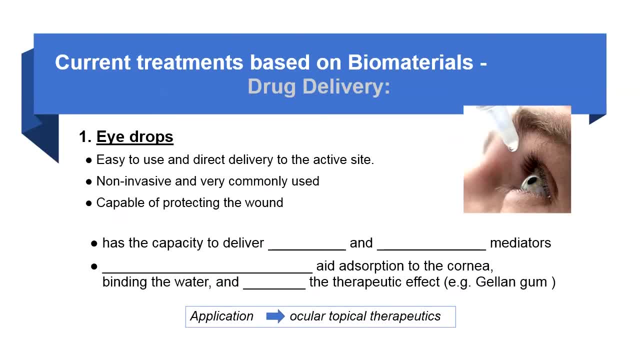 For some ocular topical diseases. eye drops are capable to deliver anti-scarring and anti-inflammatory mediator for soothing purposes. The inherent mucoadhesive properties of eye drops also enhance absorption to the cornea and the binding mechanism with water, extending therapeutic effects as a result. 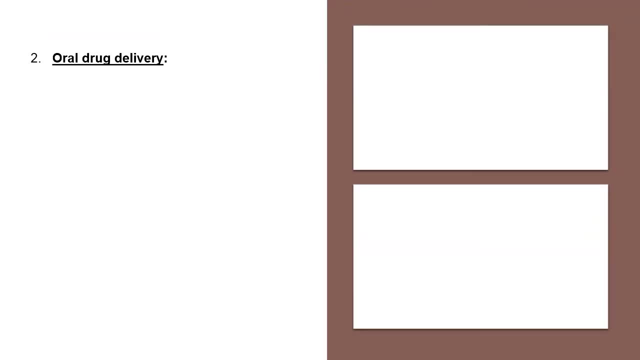 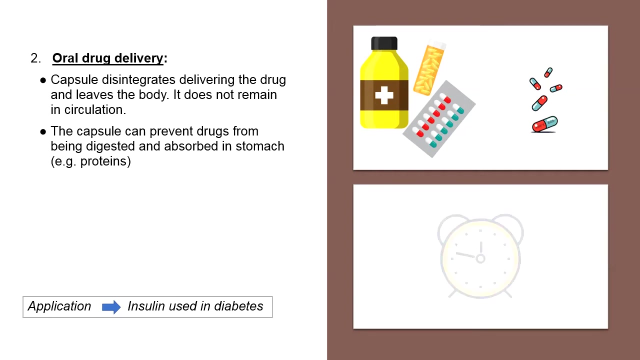 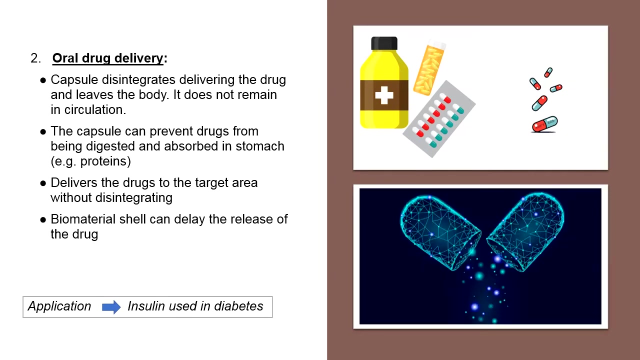 The second application is oral drug delivery. Take insulin as an example, Since insulin is a protein that will be easily digested and absorbed by our body. by introducing application of biomaterial capsules, insulin can be protected, and the features of biomaterial capsules also provide efficient time for carried material to arrive into the targeted body parts. by delaying the release of the material, 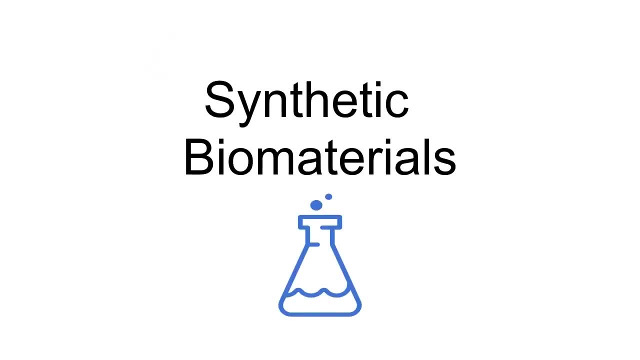 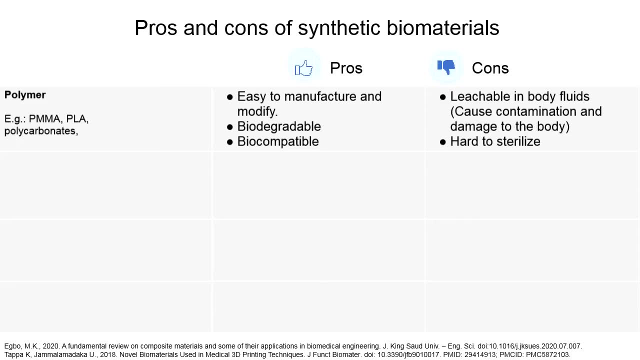 Let's talk about the pros and cons of different synthetic biomaterials. For polymer, they are easy to manufacture and modify. They are biodegradable and biocompatible. However, they are eligible in body fluids and are hard to sterilize. 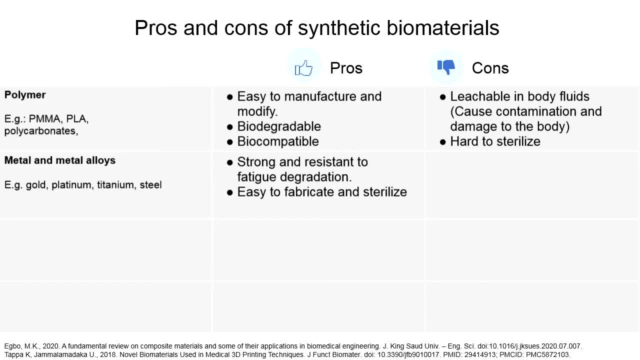 For metal and metal alloys: they are strong and resistant to fatigue degradation, Also easy to fabricate and sterilize, But corrosion and acetic loosening may occur. For composite biomaterials they have excellent mechanical properties and corrosion resistance, but they are expensive and hard to manufacture. 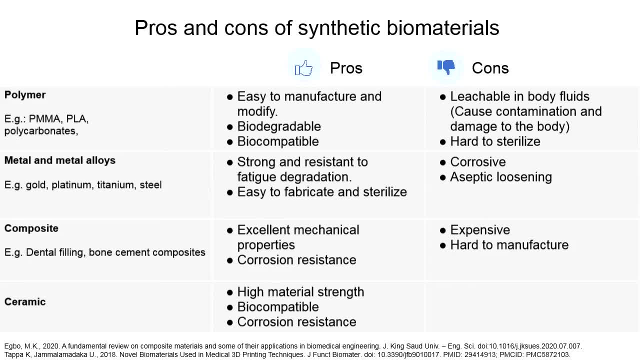 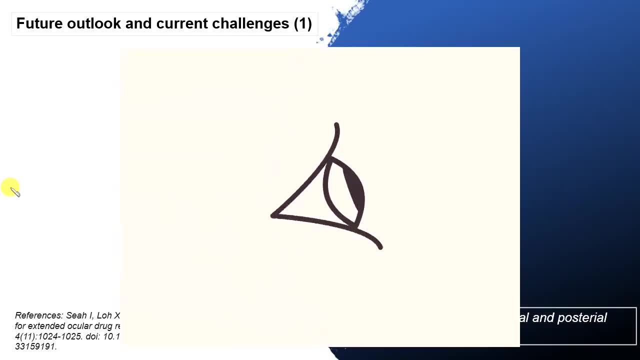 For ceramics. they have high material strength. They are biocompatible and corrosion resistant, but they have low shock resistance and are hard to mold. Many ocular conditions require patients to use eye drops, and compliance is crucial for achieving good outcomes, but it's often low. 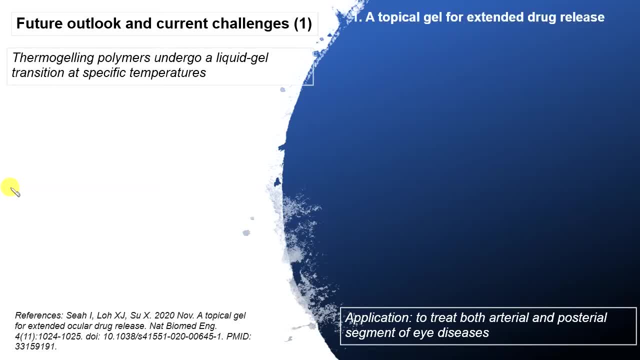 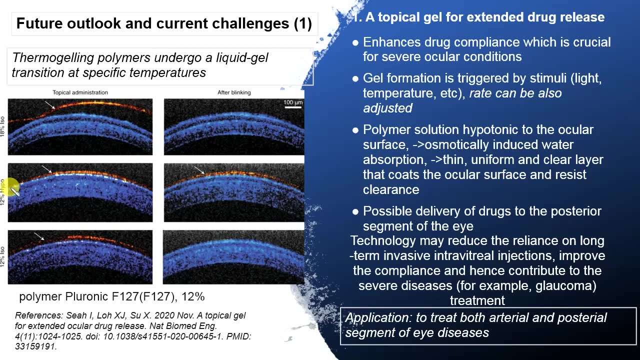 Eye drops that form a gel on the eye can help to improve compliance. Usage of polymer solution, hypertonic to the ocular surface, results in a thin uniform layer that resists clearance from blinking. In the middle of the picture you can see the hypertonic solution on the eye. 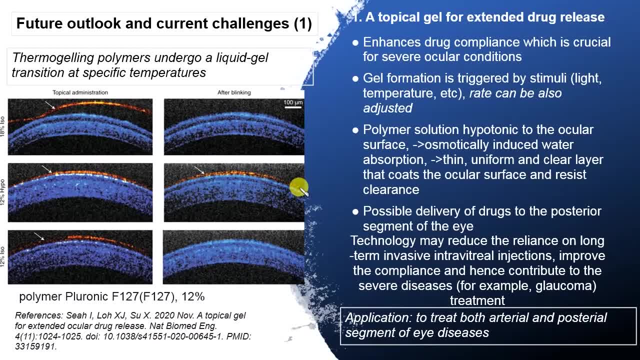 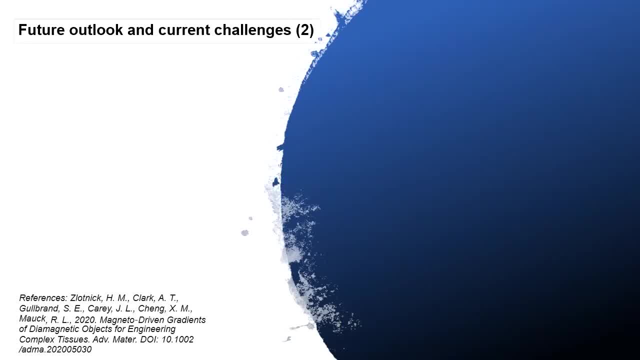 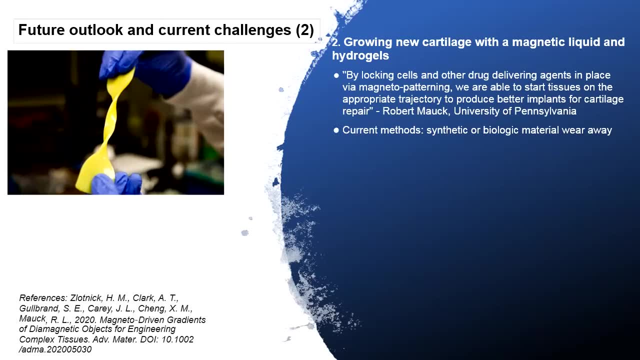 There is a layer of the solution, even after blinking. This technology also allows the delivery of drugs to the posterior segment of the eye. We also got the ability to grow tissues like cartilage. Usually, artificial cartilage wears away because its physical properties are not the same as for real cartilage. 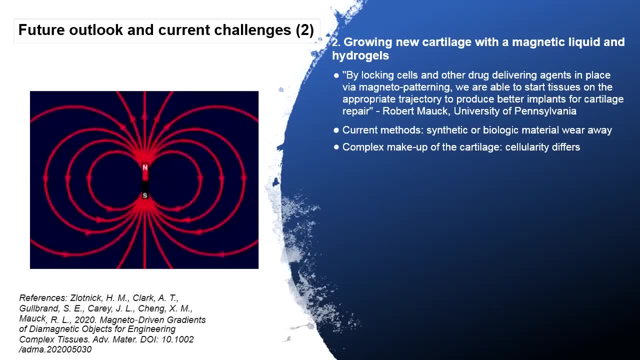 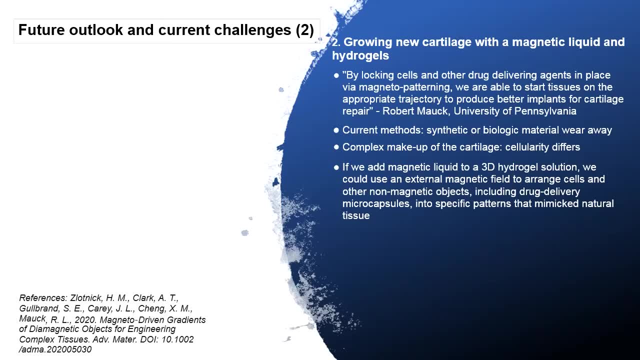 The magnetic field is used to create real properties of the tissue, for example, high cellularity at the surface and low cellularity inside the bone. Authors manipulate the magnetic character of the environment surrounding the cells. This method does not have long-lasting negative effects. 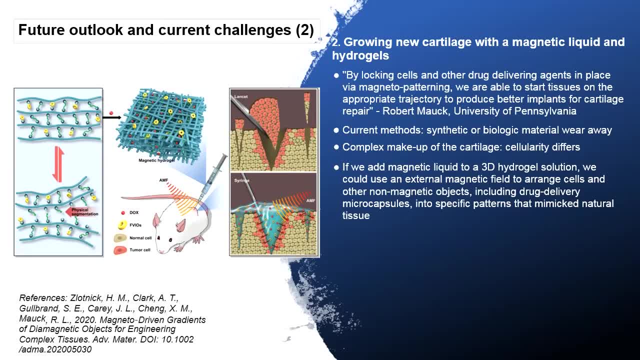 How it works. We add magnetic liquid to the hydrogel solution and use an external magnetic field to arrange the cells. After that we use ultraviolet light to fix the particles and the magnetic solution is diffused out. This way, engineered tissues get the necessary structure.